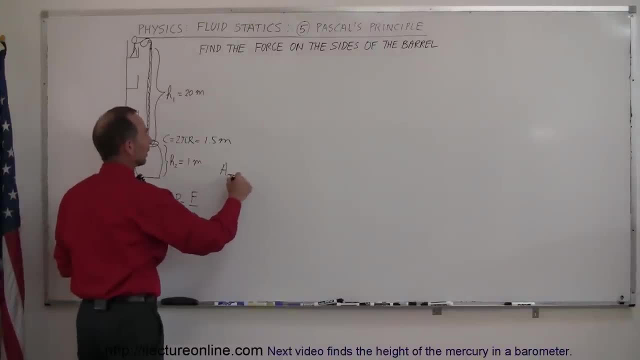 So we could say that the total area, area total- is equal to the area of the side of the barrel plus twice the area of the top, because again you have the area at the top, you have the area at the bottom and then you have the, of course, 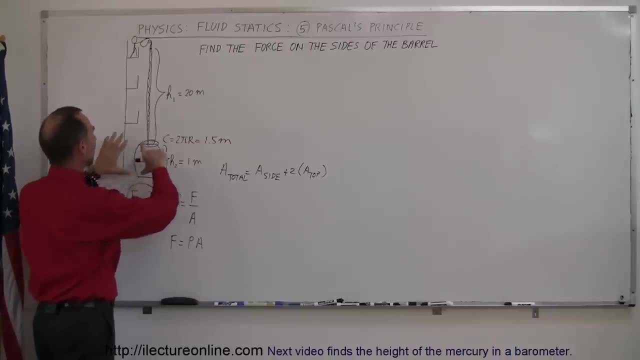 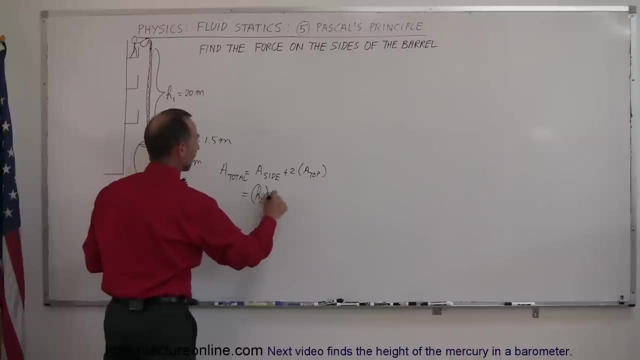 the area of the total sides and of course, the sides, is simply a rectangle where the height is h and the length is the circumference. so this would be equal to h2 times the circumference. That would be the what I would call the area of the side of the barrel. 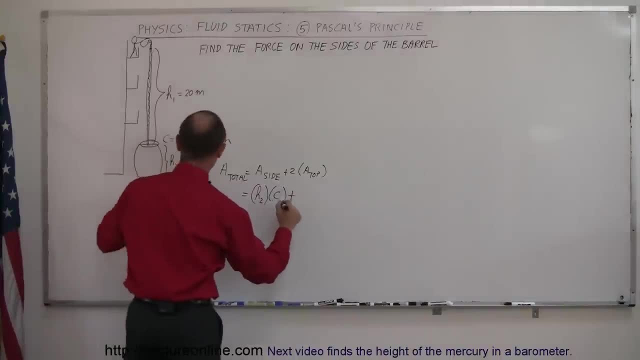 and then, of course, the top of the barrel is simply the circle. so that would be, and there's two of them, one at the top, one at the bottom, so two times the area of the circle, which is pi times the radius squared. 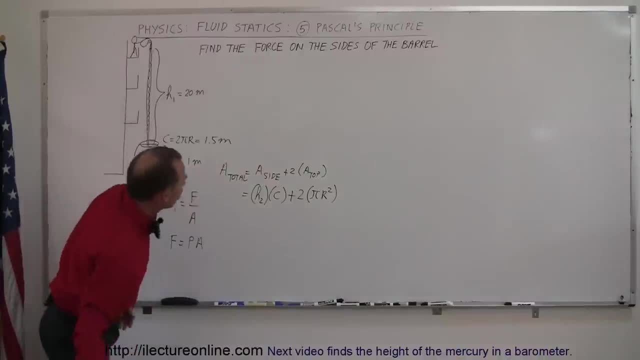 Let's see here What's the radius. If the circumference is 2 pi r, then the radius, so 1.5 divided by 2, divided by pi, the radius is about 24 centimeters. So let's say that the radius is equal to 24 centimeters, which is 0.24 meters. 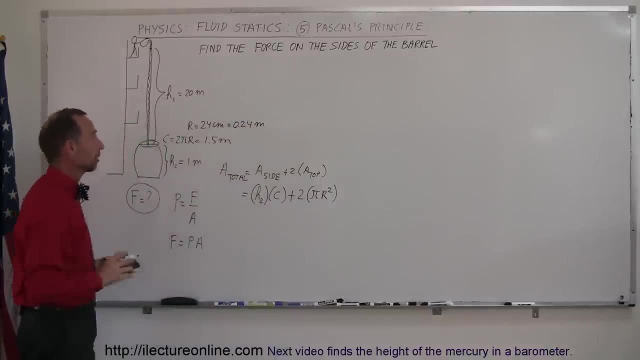 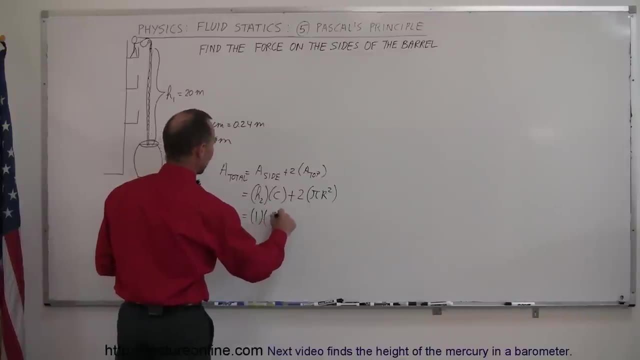 All right, now we have everything we need to know to find the area, the surface area of this barrel. So that would be equal to 1 times c And c is 1.5.. This is, of course, all in meters, plus 2 times pi, times the radius squared. 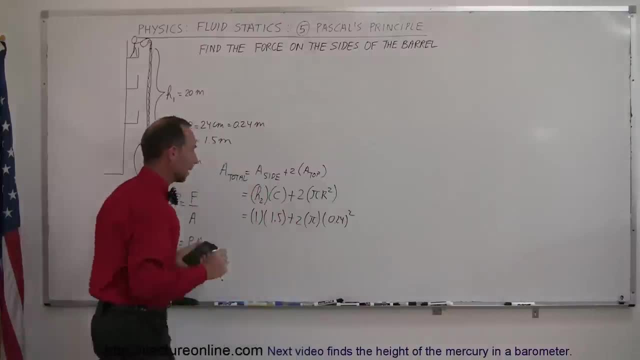 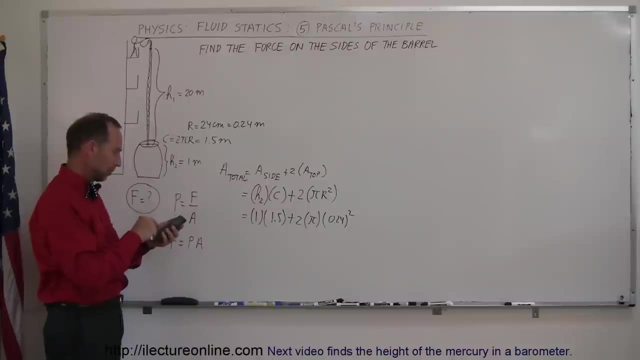 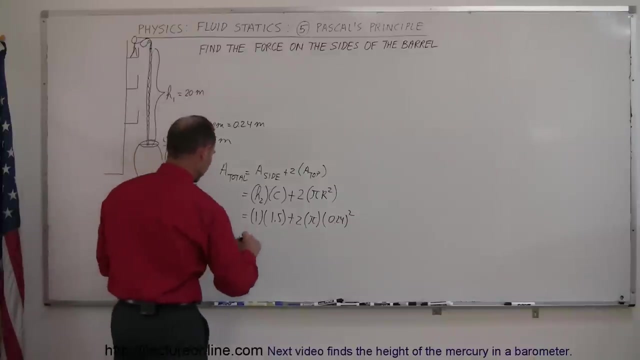 which is 0.24 quantities squared. All right. so that would be that number squared times 2 times pi, and we add to that plus 1.5, and so the total surface area area total is equal to 1.86.. 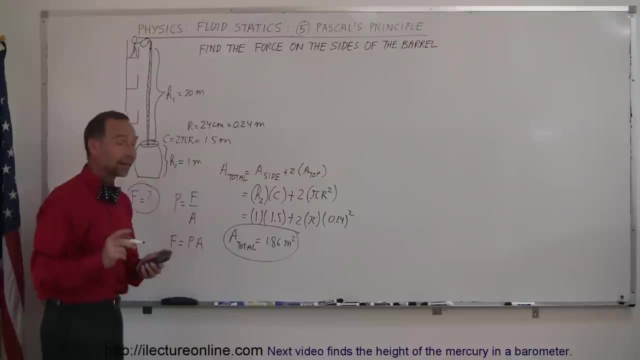 1.86 meters squared, And then we multiply that times the pressure of the fluid inside. Now the question is: what is the pressure of the fluid inside? And, of course, if we take the average pressure, which is to the middle of the barrel, 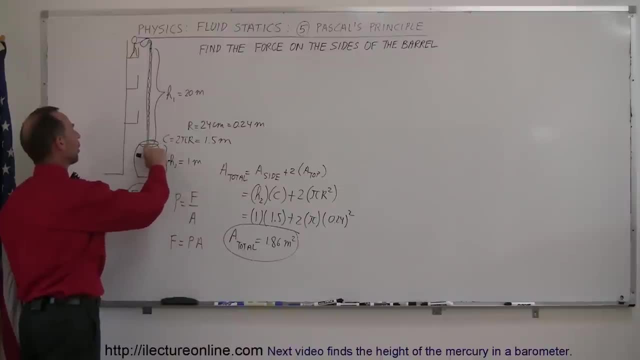 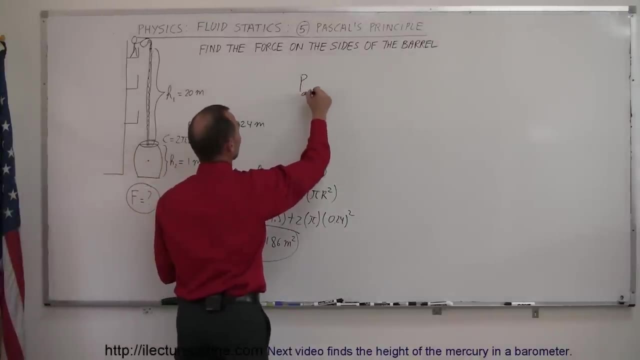 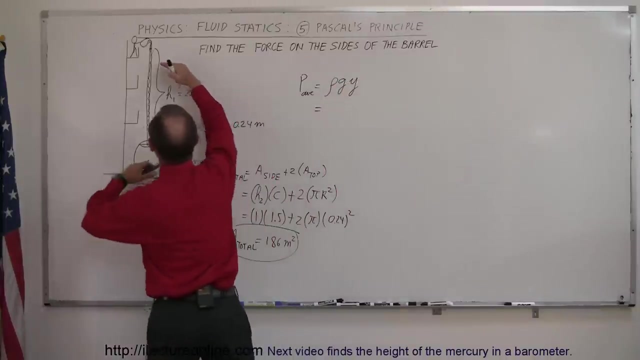 it is caused by the water above that point, all the way on the tube, all the way to the very top. So therefore, we know that the average pressure in the barrel average pressure is equal to rho g times y, And of course y is the height of the water. 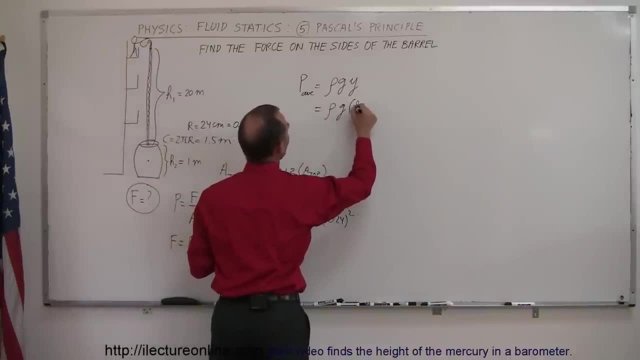 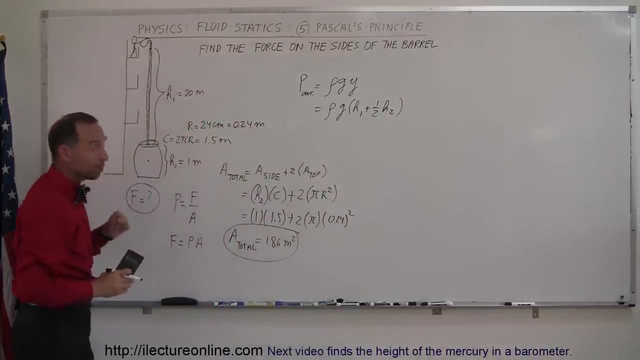 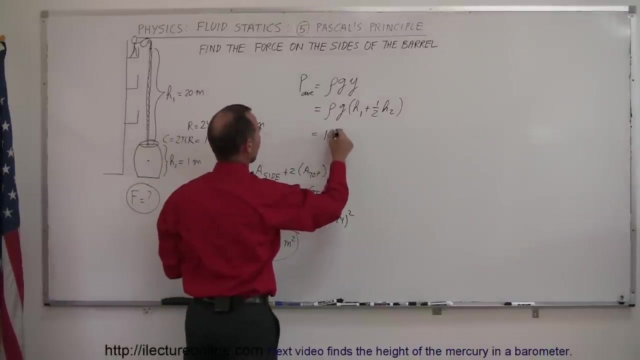 So it would be rho g times h1 plus half of h2.. Since h1 is 20 meters and h2 is 1 meter, it would be 20.5 meters high water column. So the pressure here would be rho, which is 1,000 kilograms per cubic meters. 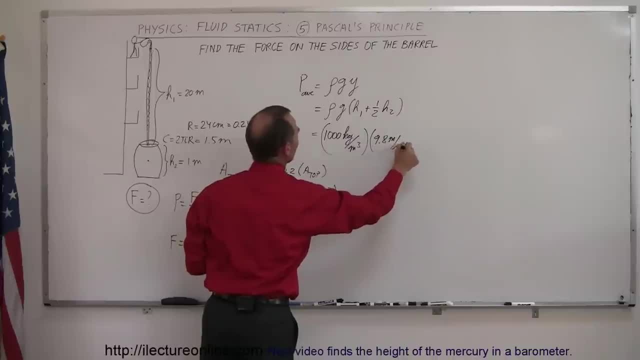 multiplied by 9.8 meters per second squared, which is acceleration of gravity, and multiplied by 20. And of course y is the height of the water column. So it would be rho g times h1 plus 1 meters, or actually a half. 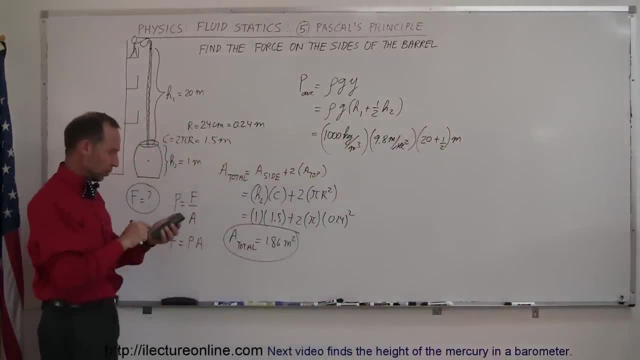 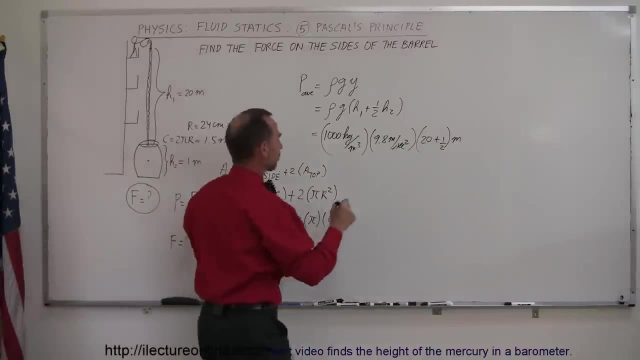 because you only want to take half the height of the barrel. All right, So that's 1,000 times 9.8 and times 20.5.. And that would be a pressure of 200,900 newtons per square meter, or pascals. 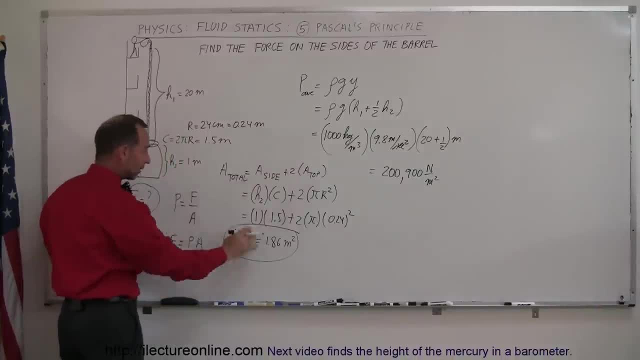 So now we combine those two. We take the pressure that we found, multiply it times the area, So the total force is equal to the pressure, which is 20,000.. Or 200,900 newtons per square meter. 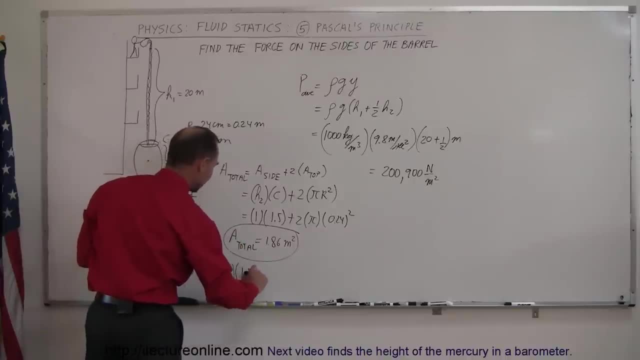 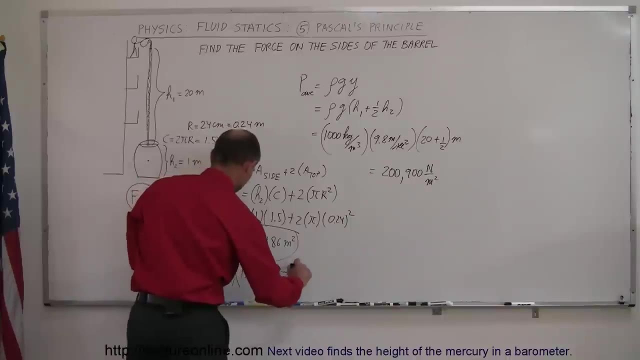 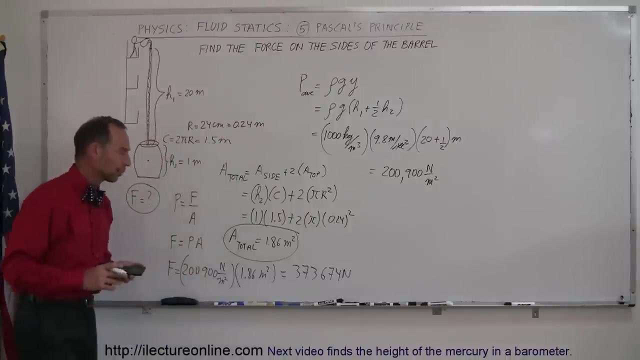 And multiply that times an area of 1.86 square meters. So take that and multiply it times 1.86. And we get a total force of 373,674 newtons. of course Way too many significant figures, but rounded off is about 374,000 newtons. 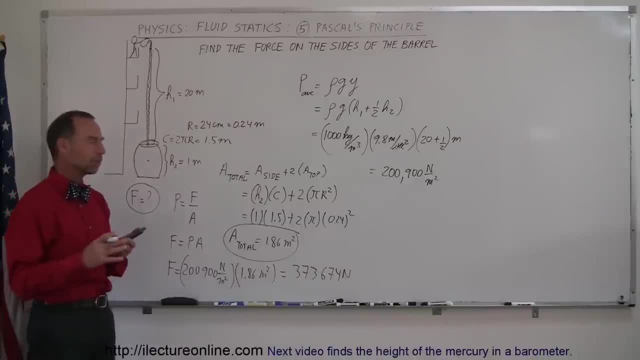 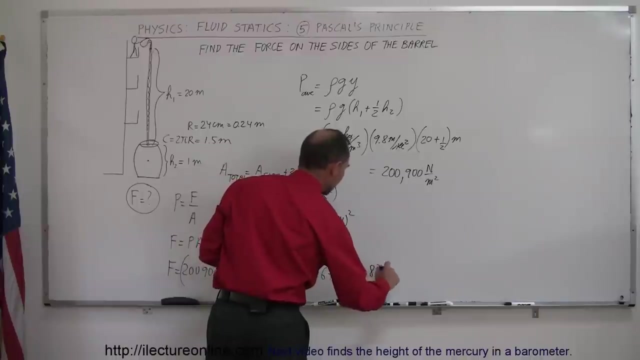 Hmm, how much is that? Because we don't have that much of a concept of how much is that. in newtons it's roughly about 4 1⁄2 newtons per pound. So if we take that and divide that by 4 1⁄2, it gives us 83,000 pounds, 83,000 pounds of force. 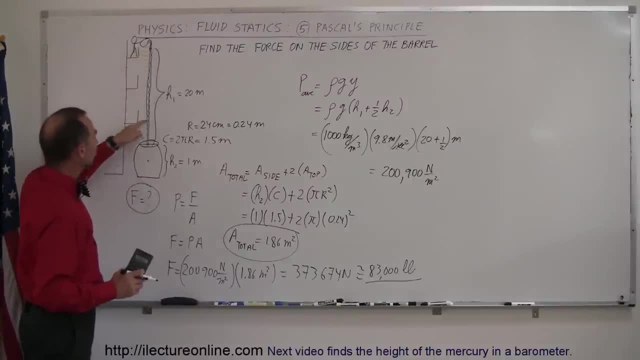 Can you imagine a small little pitcher of water filling up a tiny little tube that's connected to the barrel? if no water can leak out so the pressure is kept completely intact, We can actually create a force. We can actually create a force of 83,000 pounds inside the barrel, pushing up against the walls. 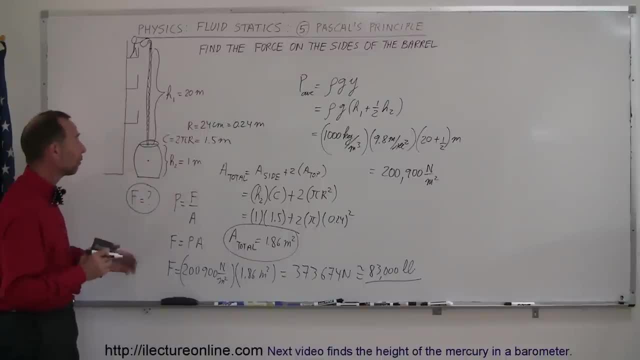 And guess what, If we were to do that? that barrel would simply burst open from the enormous force pushing down from the inside. And that's amazing. It turns out that this experiment was actually done, And I believe that the person who did that actually put up some wagers.